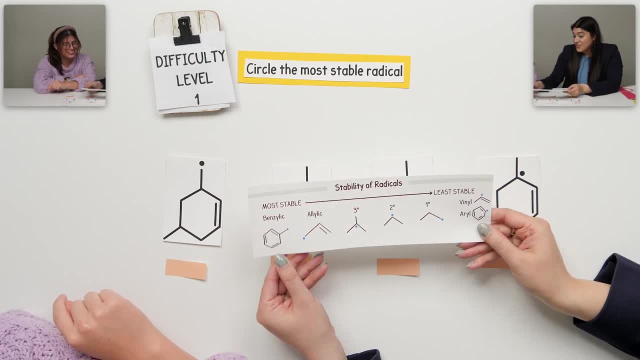 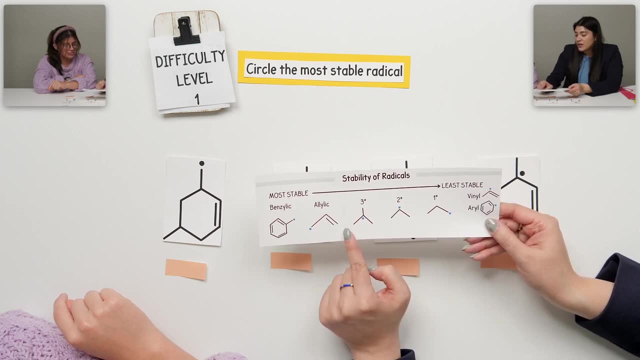 was the stability- stability of the radicals- which you said, And you know that the most stable is going to be the one that's allelic, that has a pretty much. again, it's adjacent to that double bond. You can also look at this as saying, oh, if I numbered this starting from the double bond. 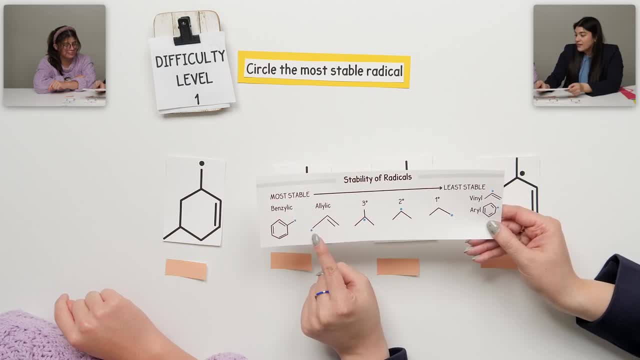 then it's going to be one, two and three carbons away. So that's really the main thing is like you're going to keep hearing that, just showing that, oh, if I numbered again this one, two and three, there's a radical. 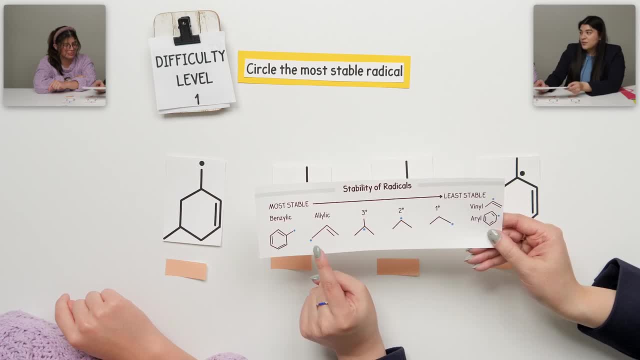 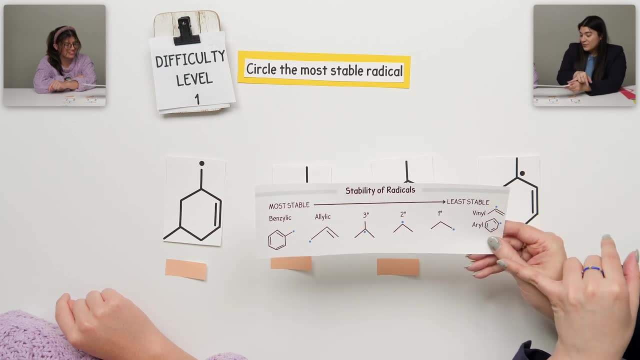 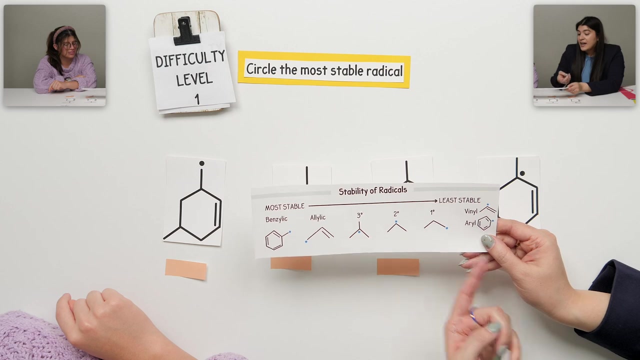 Yes, that's the allelic position, versus something that would have been vinyl, which is on the double bond that is not allelic, which you just mentioned beautifully. That would be the least stable. And then, of course, it also depends on how substituted this is: tertiary, secondary, primary and so on. 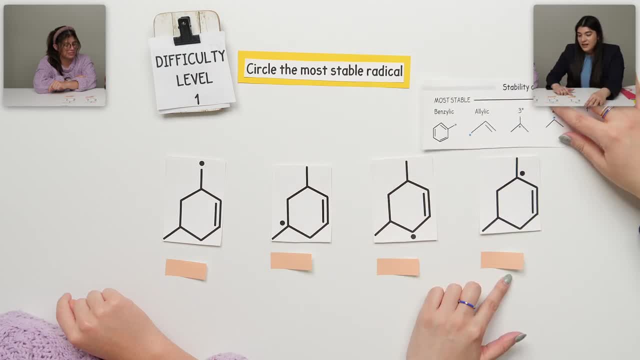 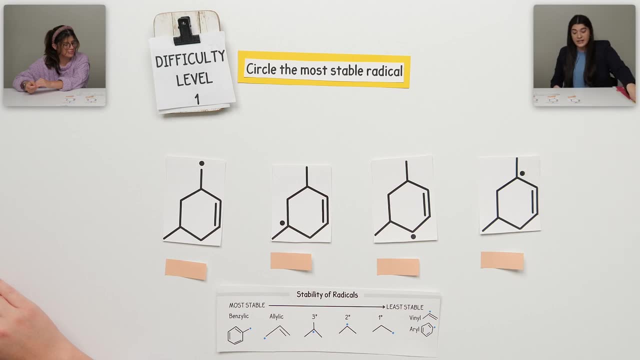 So in this case you said: well, considering these stability rules which I'll place here. I know that this guy here is allelic and it's tertiary, So I'm going to just label that First. I'm just going to say that. 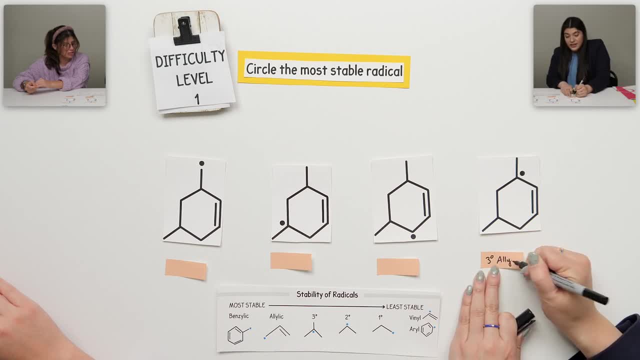 it's tertiary and allelic. This is how you would pretty much define what this is. And then what would this be defined as Classified? This one right here, Secondary Good, And you also mentioned. yes, it's allelic because there's one, two and three. 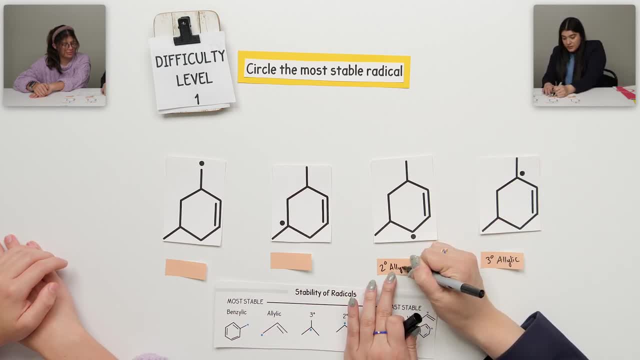 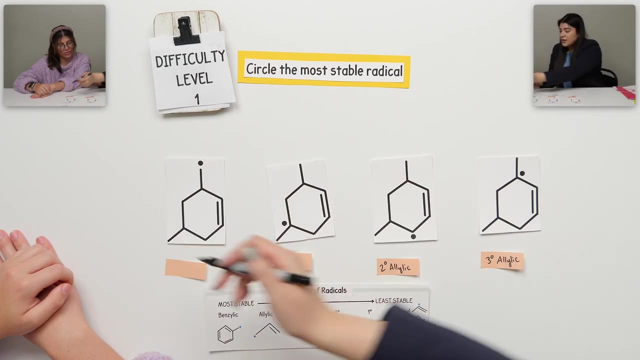 That separation? Yep, This is also allelic. How would we classify this one? This one would just be tertiary. Is that right? Because it's just on this one. So one, two, three. Good, That one would just be tertiary And this would be primary. Let me write that I know that's. 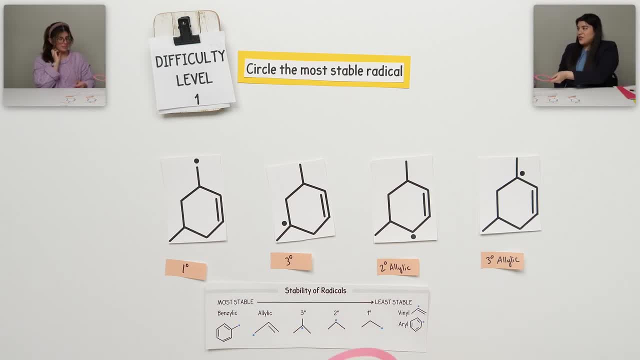 the worst. We already said that. okay, if you want to do the honors of circling, the right one, that's it. And of course, I just want to just show the classification, for you went right to allelic. I know that it's going to be the most substituted, which is beautiful. 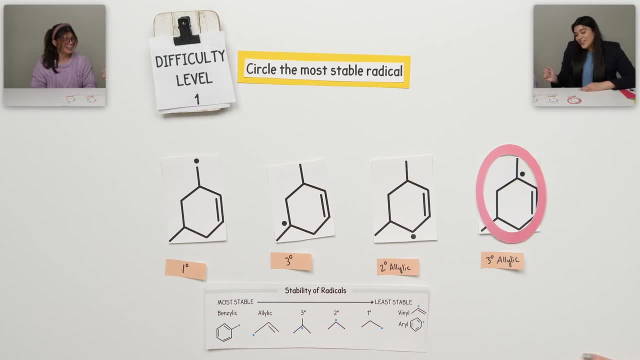 You do want to do this quickly on an exam, you know, and this one was like: okay, this one was like an easier one, right Difficulty level one, That's one that it's like, for sure, know it So great, That's it. I know tertiary allelic Yep, This is the best one, Lovely, Lovely. 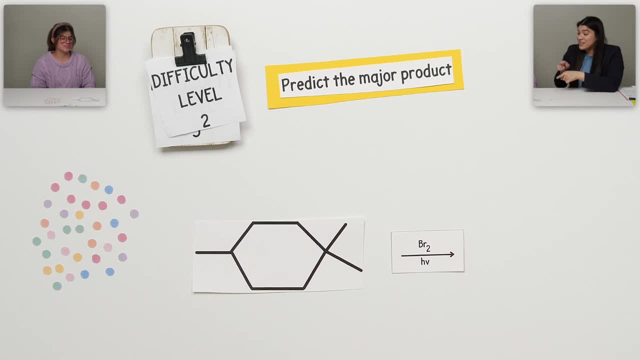 Okay, Off to a great start. So, moving up to difficulty level two, we're going to predict the major product. Yes, And remember, with radicals, there are several possibilities. Yeah. However, we still go back to what we just looked at: stability, picking what was going to be. 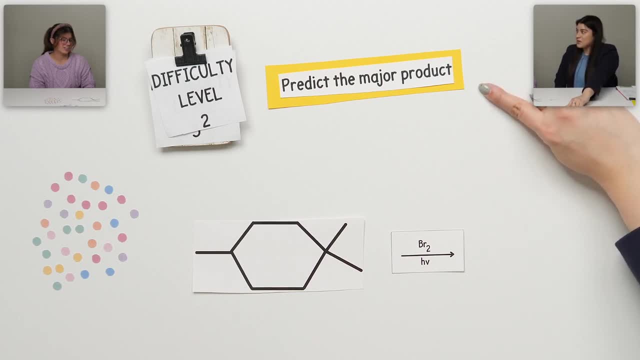 the most stable And you know that's going to define what our major product is. So what do you think our product, our major product, would be in this case, And why It would have to be? What kind of radical option do we have? And we can place them with different colors. 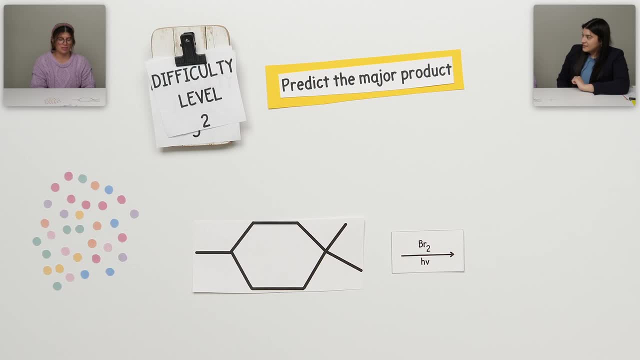 just seeing the different options. Okay, So it'd be, we could do. I guess we'd have a few Good So we could do, not this one, because that already has four, But honestly we could do like all of these ones, but they're kind of just the same Good, So 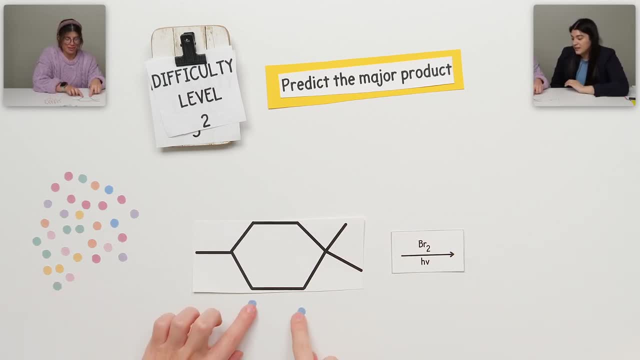 with the same colors. let's put them accordingly. Okay, Now would these two be the same? Oh wait. no, they wouldn't be, But these ones would Wait. these ones would Good, And then these ones would. 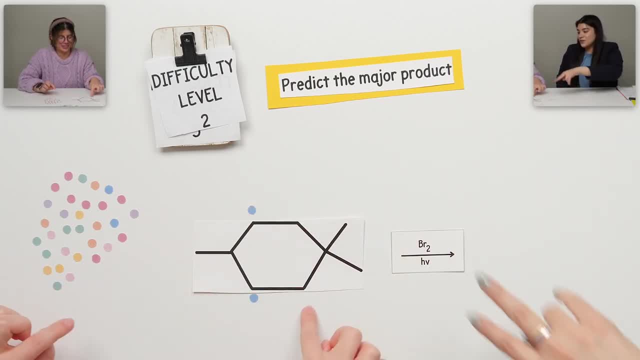 Yes, And it's based on what it's next to the substituents. Good, Those, both are on by the methyl, And then this one right there, And then we'd get a tertiary like a tertiary right there. Okay, And that's the only one that's tertiary. That's the only one. 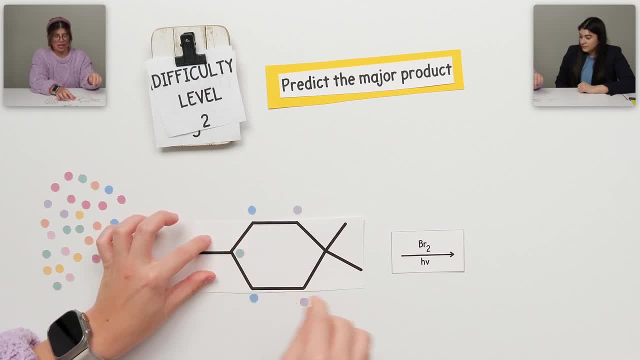 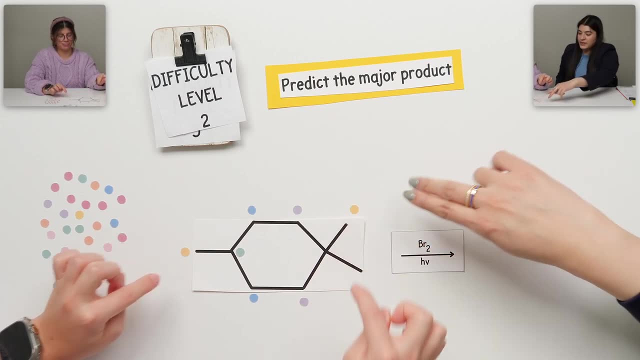 And then do this one, And then we have a few like primary ones. Okay, So these guys right here, But these two wouldn't be the same, correct? So just that. Oh yeah, because this one's attached to the four bonds, Do orange. 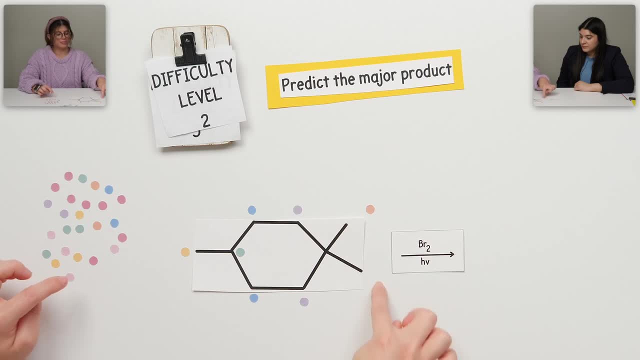 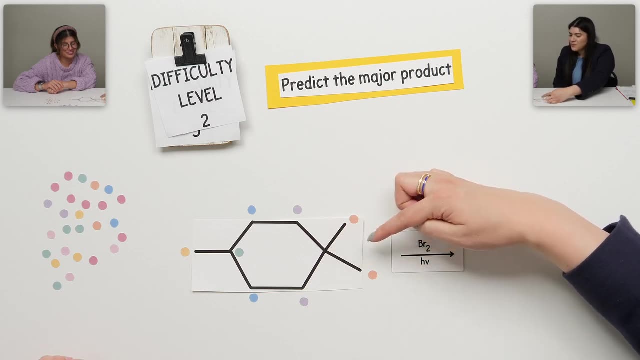 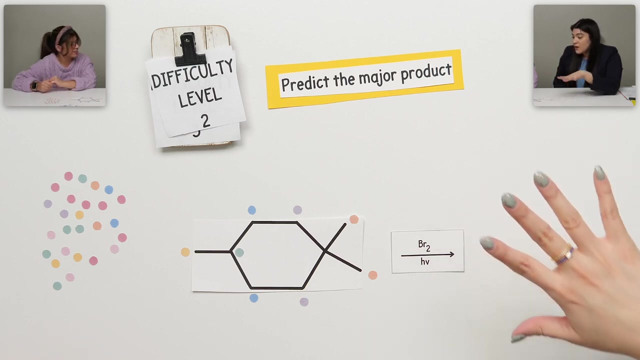 Like that Great. I loved that you were not fooled by this. A lot of people would have been and said, oh, I can place it pretty much at any carbon. That's not true. You can only place or have this radical form when there is a hydrogen available And that. 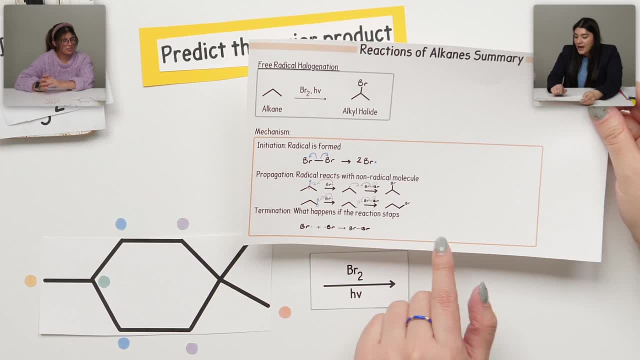 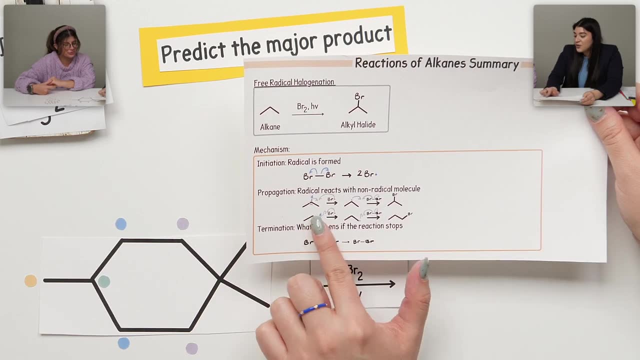 all goes back to the mechanism, right. So, going back to specifically our propagation step, where we are combining that radical with a non-radical molecule and it's taking it from the bond of the hydrogen. So that's why hydrogen again had to have been available to us. 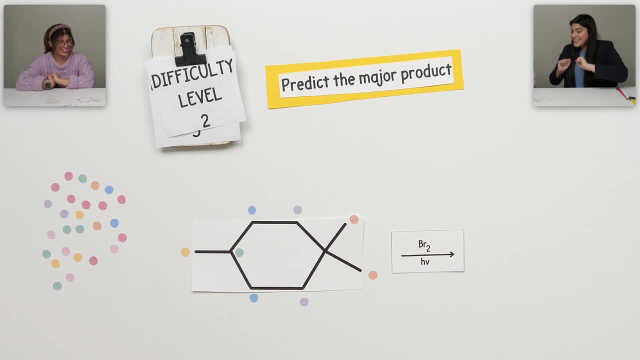 So great. I love that you got that right so far. Next, what is going to potentially be the major product Like which radical would we pick from? I would say this one. Why? Because it has the tertiary Beautiful Yeah. 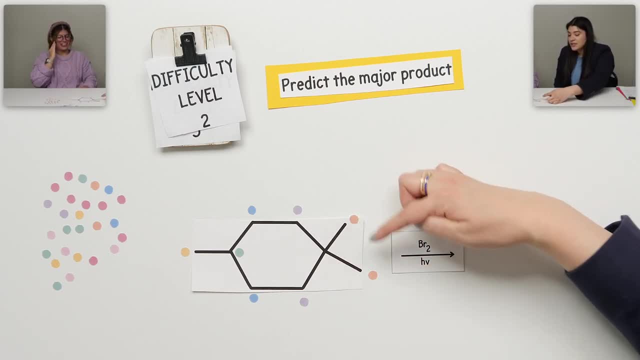 That's why. That's exactly why- And you named it here as well- You said that these are primary, So that's the weakest, That's not the most stable, So it's not going to produce the major product That would have been a minor product. 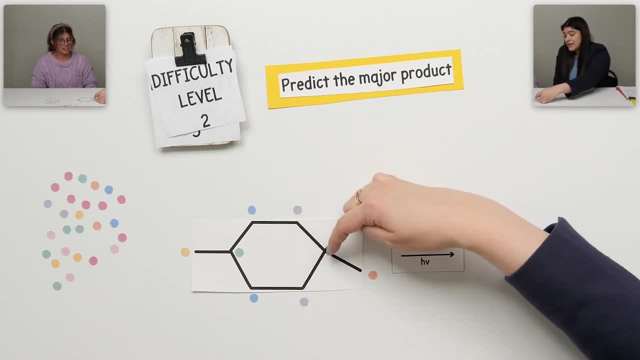 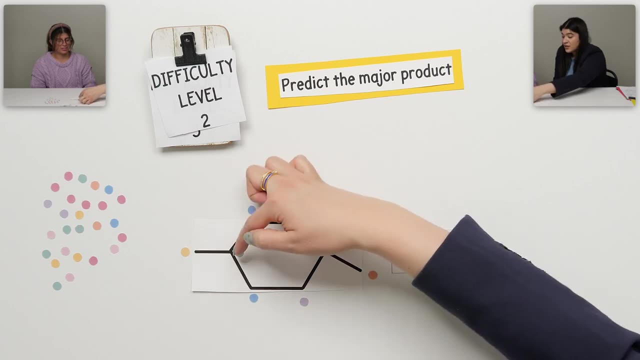 Yeah, Then I know that these are secondary because they're attached to two other carbons, Same with these. That's not the best one. The best one would have been tertiary. It's attached to three carbons, So great Okay. 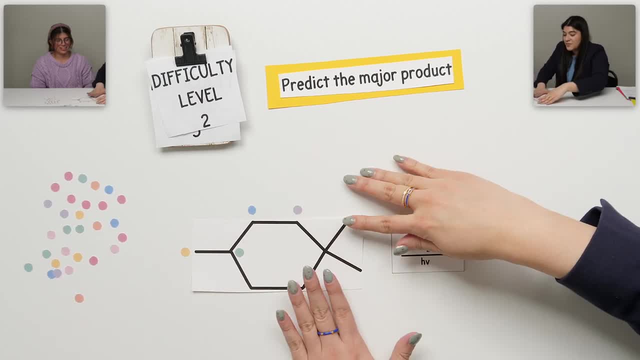 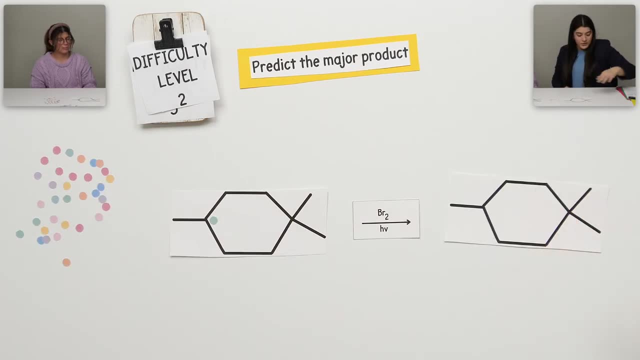 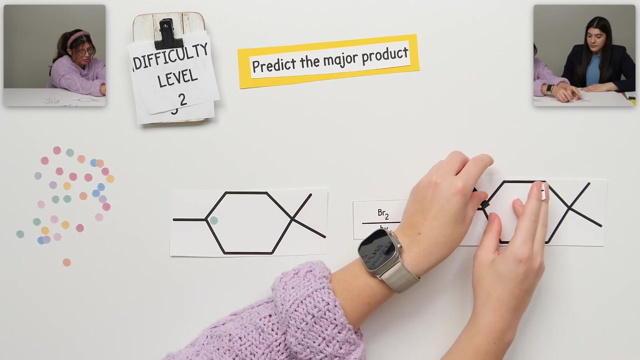 I'm now going to say: forget those, I accounted for them, but that's not the best option. The option I'm choosing is going to be the tertiary one, Right? So let's draw it out, Let's build our product. So now I'd be. we just basically replaced the radical with the halogen and look like that: 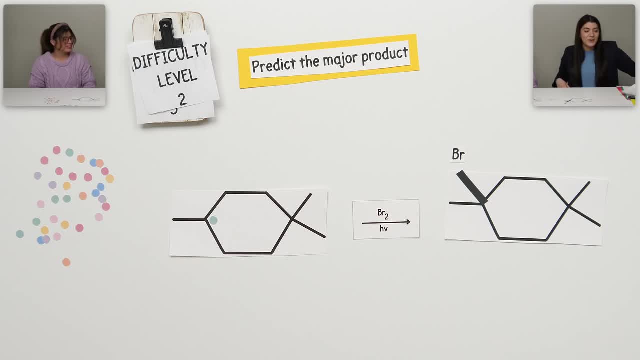 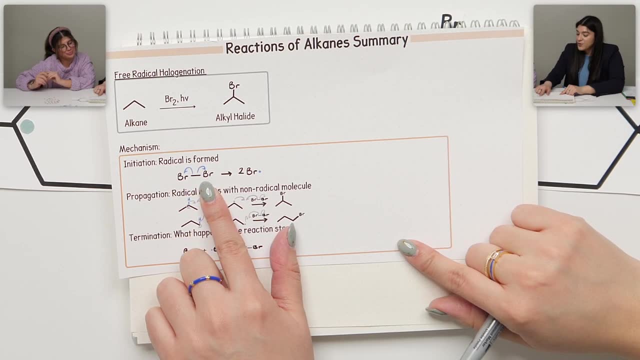 It would look like that. Perfect, That's it, And it's again going back to this mechanism. just knowing that I already formed, I did that initiation step. right, I did that initiation step, I formed. the radical Actually ended up forming two. 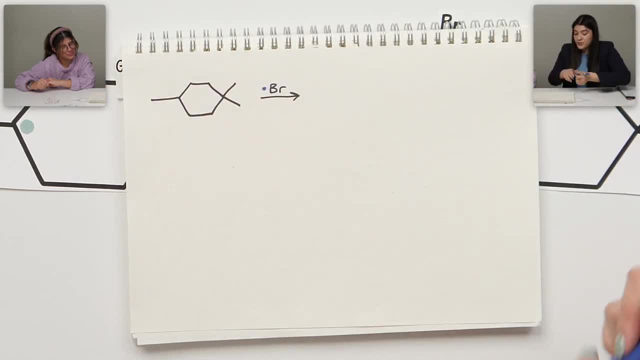 I'm now going to use that radical and specifically this tertiary position I'm taking from the hydrogen that has to exist there for me to even continue this reaction, And that's where I'm taking an account for both of those electrons, doing that single headed arrow. 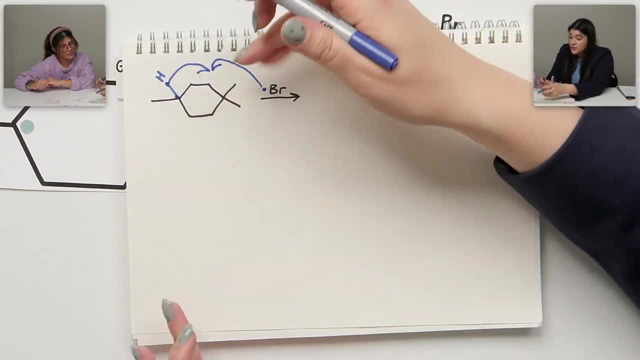 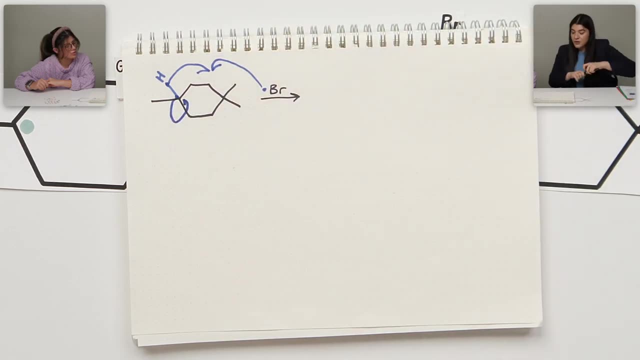 That's how we're going to end up forming this bond. Actually, the first step is still going to be forming that, the radical that we just did here. So this goes back on to that carbon. I'll draw this out again, Like it's possible that you might be asked to show the mechanism. 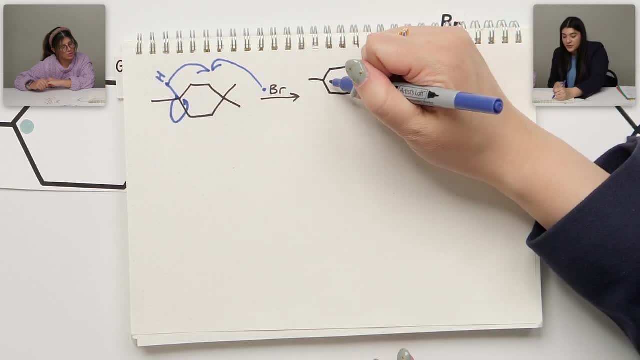 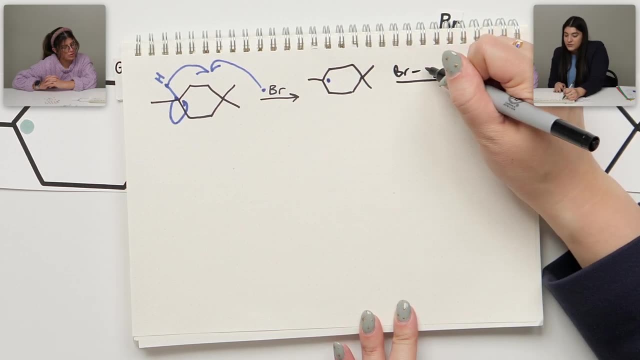 I know that this electron now moves here And I Form my radical. We have not added that bromine just yet. Instead, this is where the step goes from. We still have again two bromines that are attached. This is where we're going to add on that bromine.